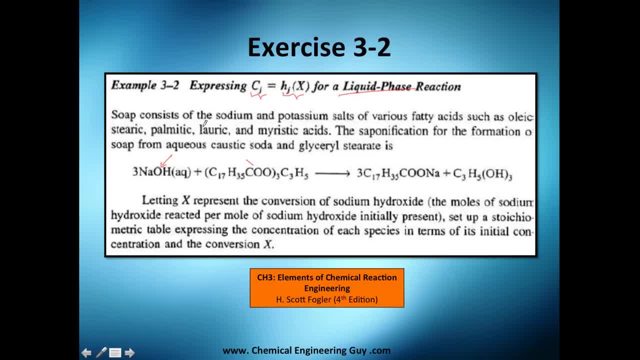 everywhere of various fatty acids such as oleic starch, palmitic, lauric and mystic acids. This is a pontification for this formation of soap from aqueous caustic soda and the glyceryl stearate here. Let X be the conversion of this sodium hydroxide. this guy here. 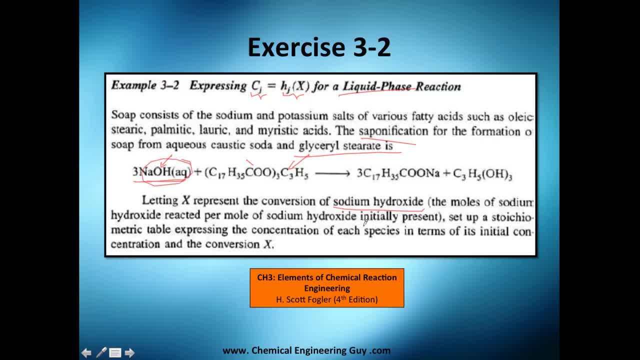 the moles of sodium hydroxide reacted per mole of sodium hydroxide initially present. set up a stoichiometric table expressing the concentration of each species in terms of initial concentration. Okay, initial concentration of A and conversion of A. Nice, You can find this. 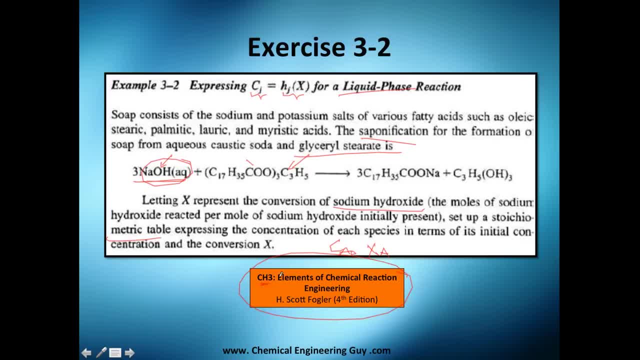 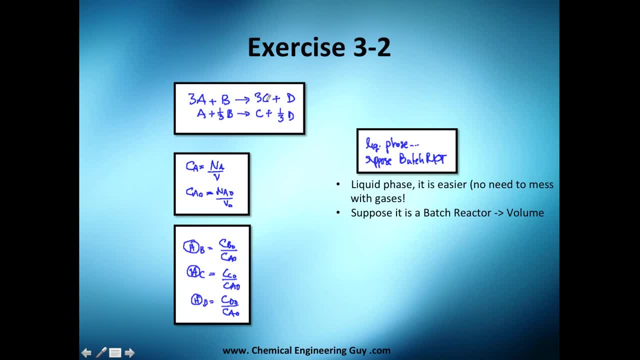 problem or exercise in this book, chapter number three, Let's do it First thing first. we got this reaction: Three times A plus one mole of B will give you three moles of A, So one mole of C and one mole of D. Since they are asking us to do it in the caustic soda or 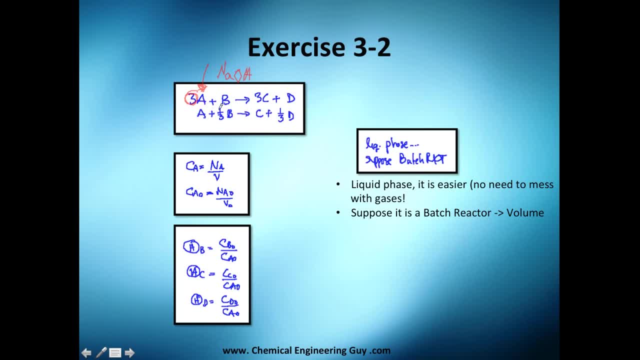 sodium hydroxide. we need to get rid of these three. So let's divide it by three. everything, We get one one-third. one one-third. Good. Now we are in liquid phase, so it's easier. We have 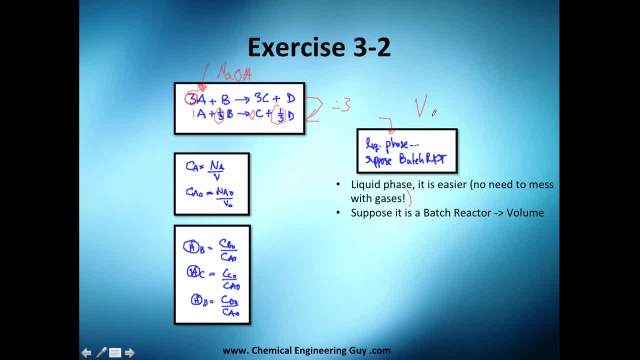 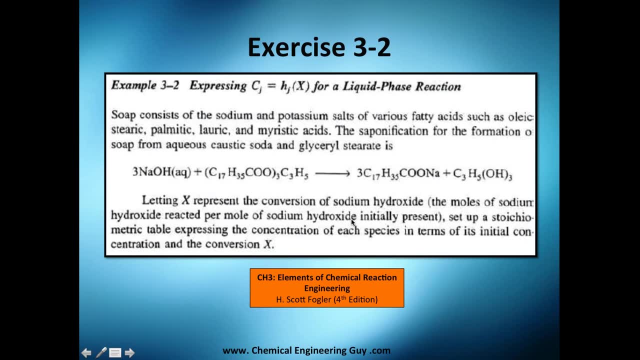 we don't need to mess with gases and our volume is constant. Initial volume equals final volume And I'm going to suppose it's a batch reactor, because I have no clue. They don't tell you anything about what type of reactor is, So I'm going to suppose it's a. 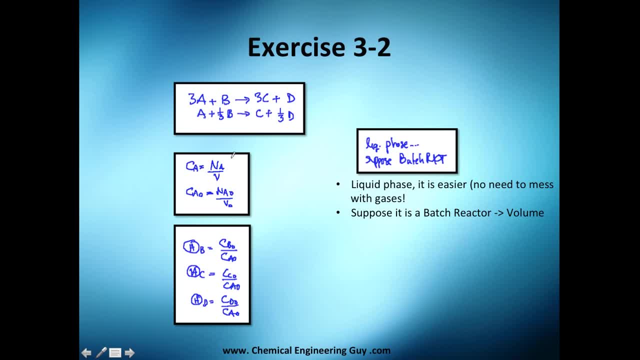 batch. So by definition, in the batch reactor, you know, there's no inlet, no outlets, only accumulation, yeah, only accumulation and consumption generation here. So concentration at any moment is total amount of moles at any moment divided by volume. 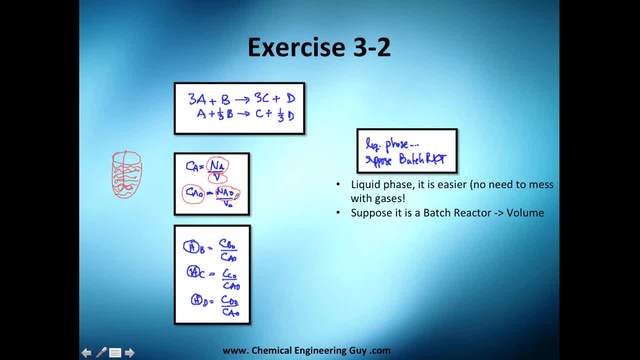 Initial concentration of A equals initial moles of A at initial amount of volume. So just one thing I want to tell you here is that these volumes are the same because it's liquid phase. Now let's check this function out. The H circle of B, C and D is just initial amount of. 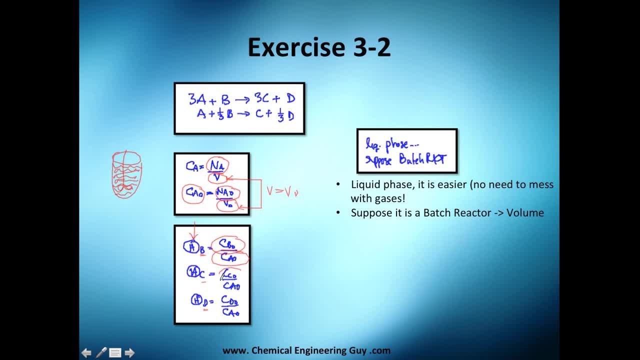 the concentration of B divided by the concentration of A. initial amount of concentration of C divided by the concentration of A at the beginning, and the same for D here. So you can see, probably is this here divided by. so, since the volumes are the same, probably you are asking yourself why. 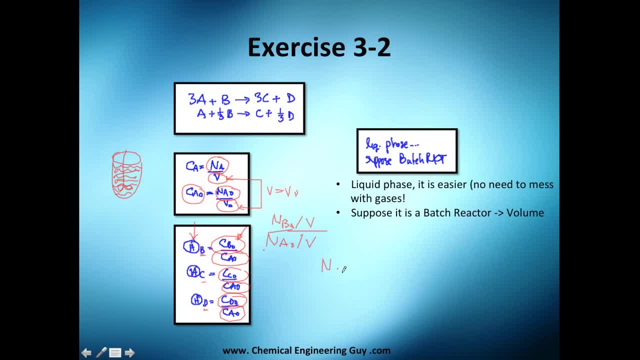 are you using this definition if we tell or we were asking… Here, We got this before. This is the H circle function, any value. so why are we using concentrations? because I just multiply and divide by volume. so you know, this is definition of concentration and this is. 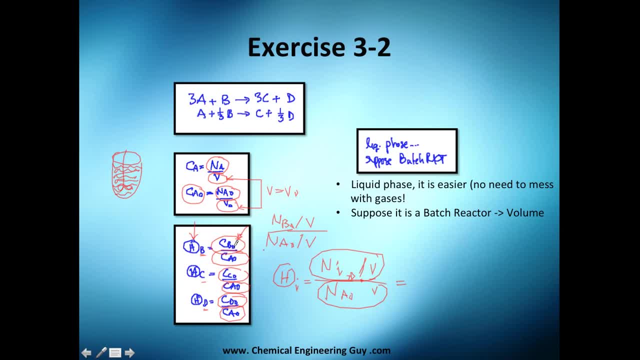 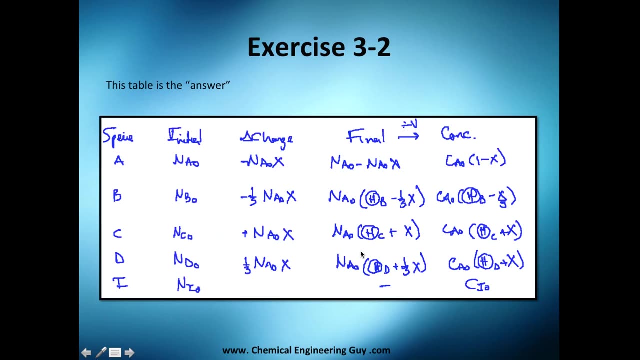 definition of concentration of A. so hopefully you don't get lost on why I use this rather than moles- it's the same- because I'm divided by a volume. each of these volume and volume mathematically is one. so yeah, let's continue with this. let's calculate this table. you know this table a little bit, so the initial 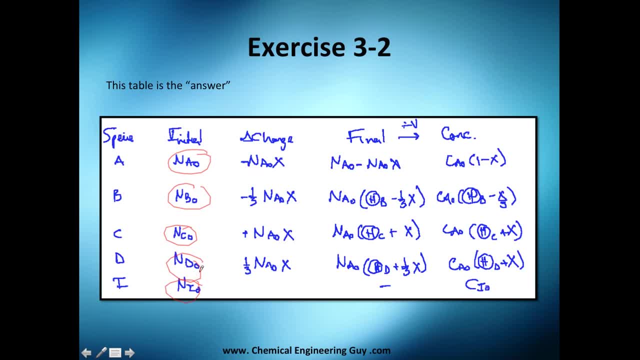 amounts. we have them here here and here here as variables. the changes: well, this is A, which is 1, and this is B divided by A. A, remember, is 3, B is 1 minus 1. third, this is C. divided by A is 1. divided by 1 is positive 1 because it's A. 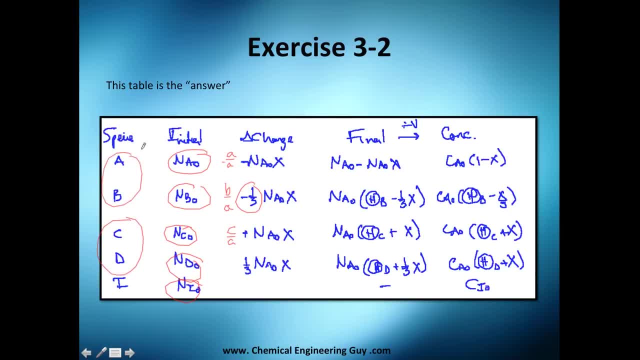 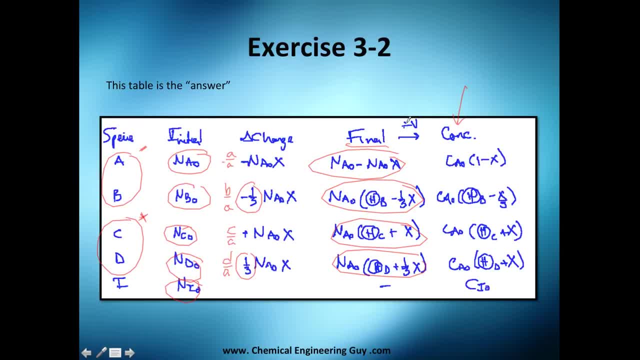 concentrations. well, we call just divide by volume here. divide this by volume and you will get the concentration. divide this by volume and you will give the concentration. divide this by volume and you will get concentration. and divide this by volume and you get the concentration. and once again, we got this in terms of initial concentration of A. 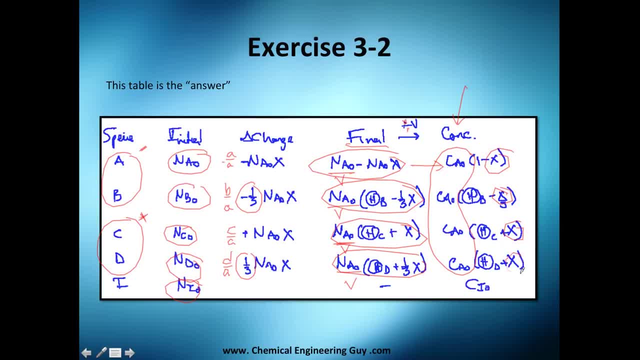 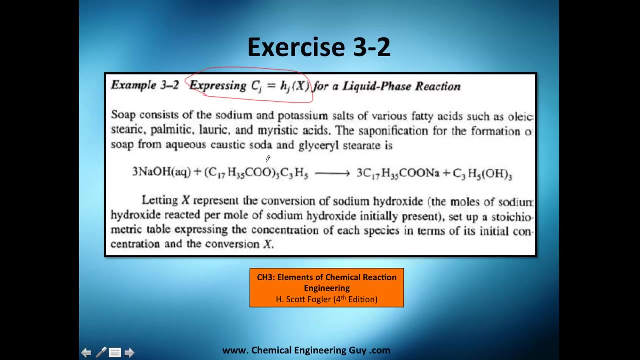 in terms of conversion of A, and this is the terms of, or the reactants, B products, C and D. but we respect with the moles of A, so we're done. this will be the table on A's with the result A and D that they ask us. they tell you to do a express these in conversions, and where is it? 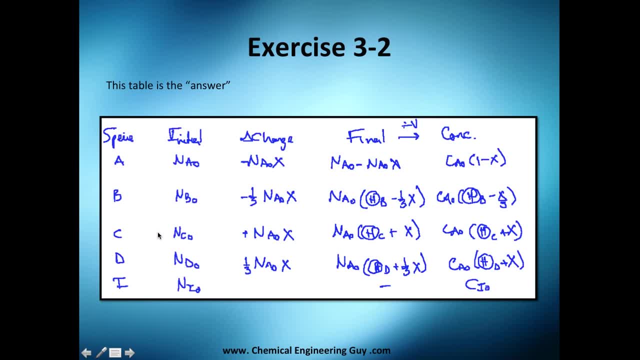 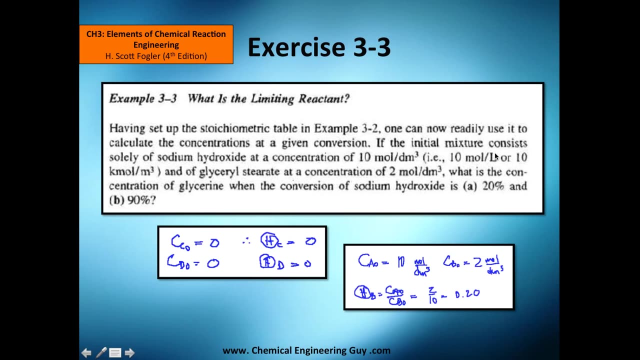 set up a stoichiometric table and this is our stoichiometric table. so that's exercise three. essentially, the only difference is we got this value here. this is one, this is one third, and yeah, that's everything, guys. see you in the next exercise. i will break it so you can understand it. 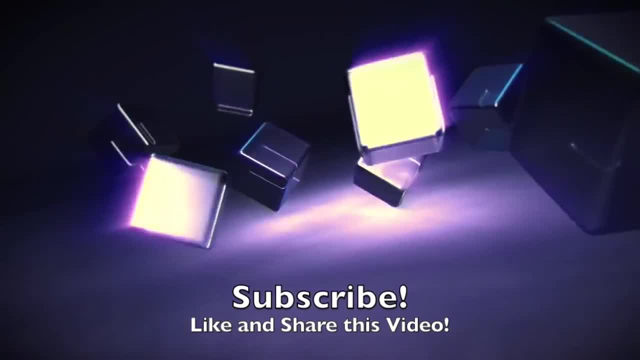 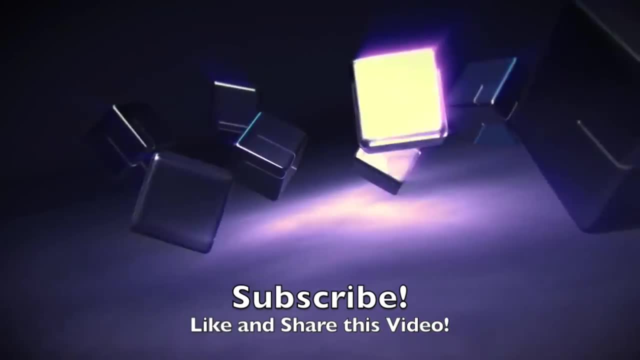 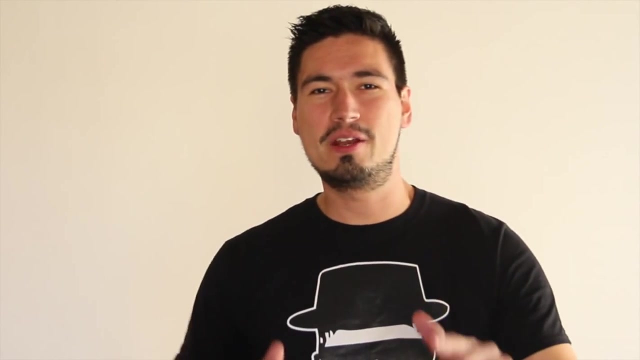 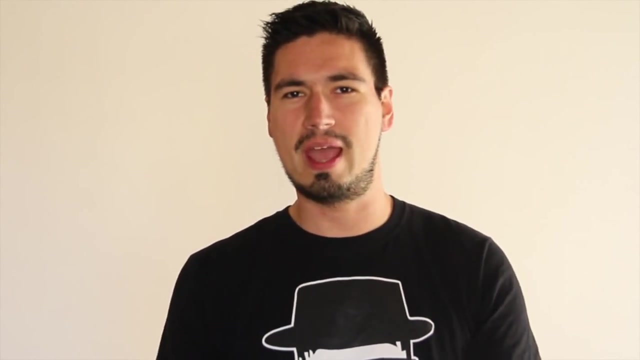 easy. what's up guys? it's me chemical engineering guy. so if you like the video, why not push the like button? it really helps me to know if you're liking the videos or if i should be changing something or i should be adding something, taking out content, whatever. also, sharing is caring, so if you got, 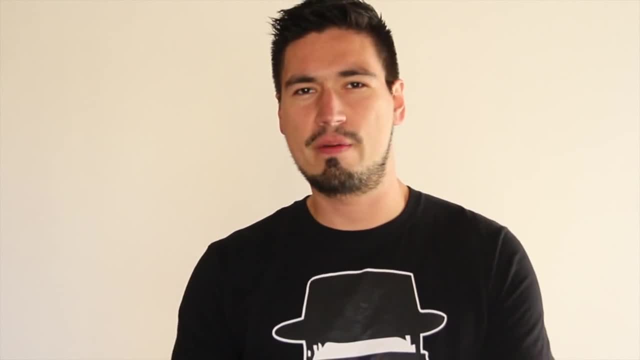 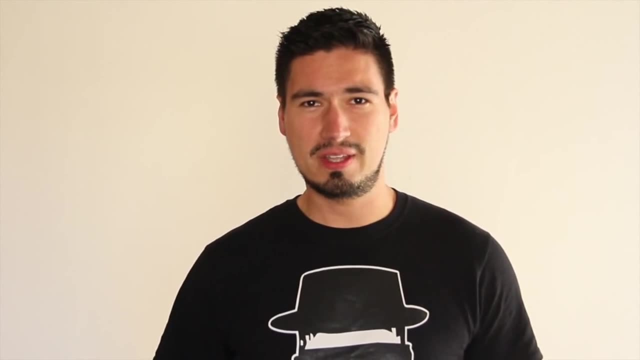 the video. please like it and subscribe to the channel if you want to see more videos like this. any kind of friends, teachers, colleagues or whatever kind of person that might be interested in this type of content, why not share it? sharing helps our community to grow faster in members and 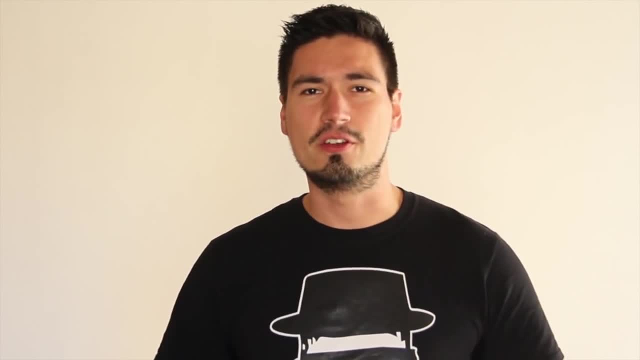 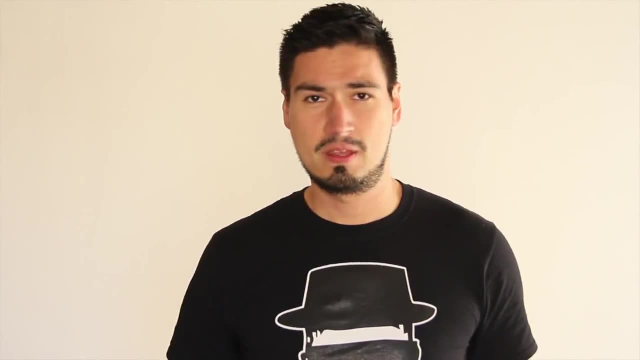 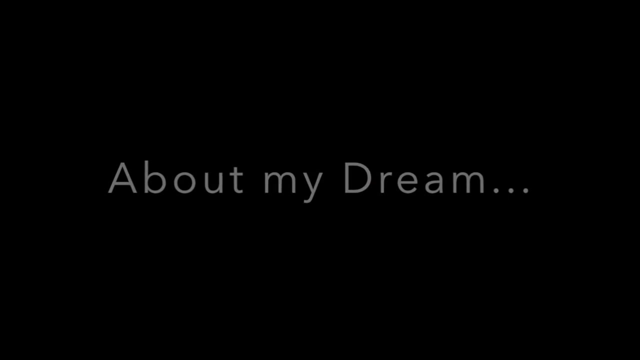 in content. if you want to keep track of my activity- videos, uploads, experiments, plays, whatever content i'm getting youtube- be sure to click the subscribe button. subscribing to the channel is totally free, guys. my dream is to create an online academy of chemical engineering where everyone can access it in the world. 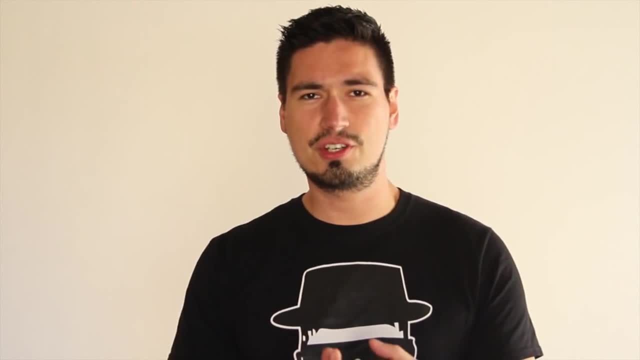 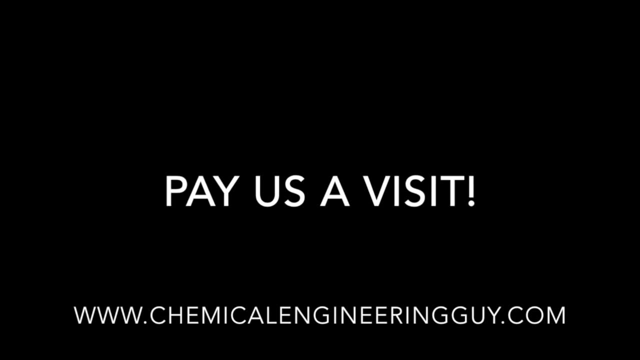 imagine a place in which the student, the teacher and the engineer get the best of each other. so thank you, thank you, thank you, guys, for the support and the love.